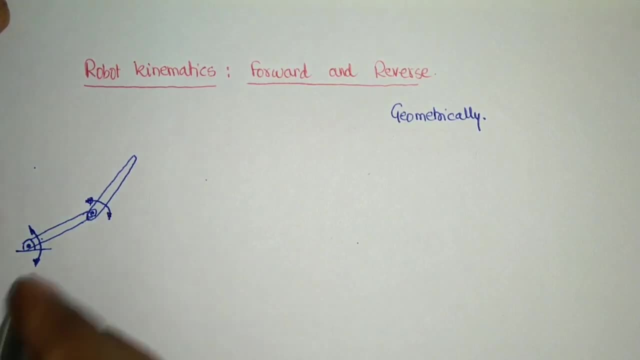 And as we discussed in our notation part, and as we already know to some extent, that this will be given by this theta 1.. So theta 1 is the rotation associated with the link 1.. And theta 2 will Will be the rotation associated with link 2.. 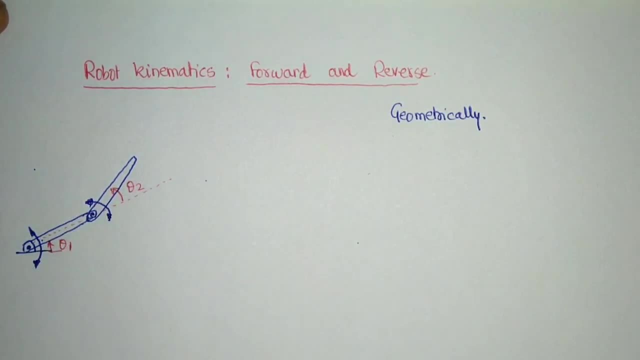 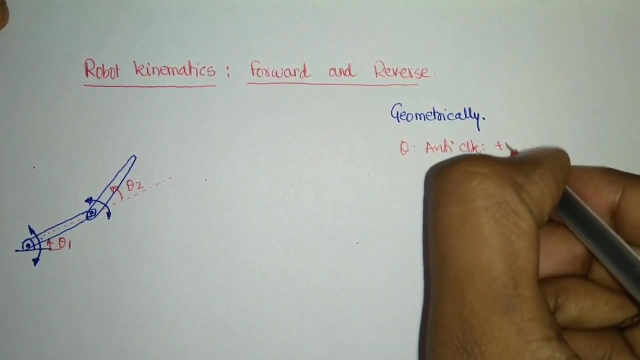 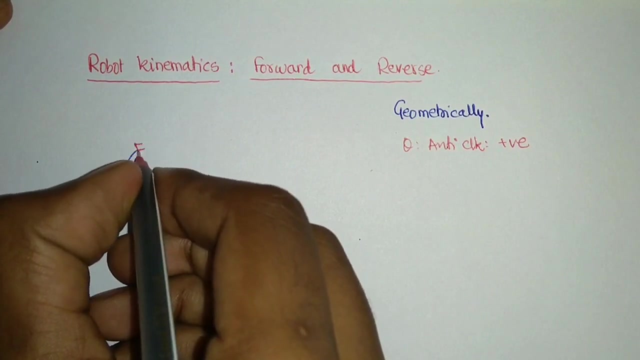 Okay, So this is my theta 2.. Okay, Theta in anti-global direction we take as positive. Okay, So theta in anti-global direction will be considered as positive for our analysis purpose. Okay, So if this is my end effector, right. 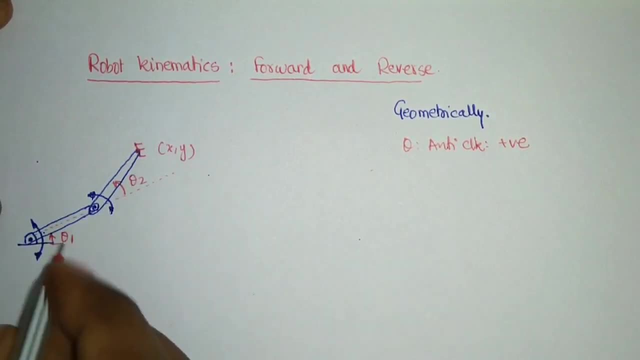 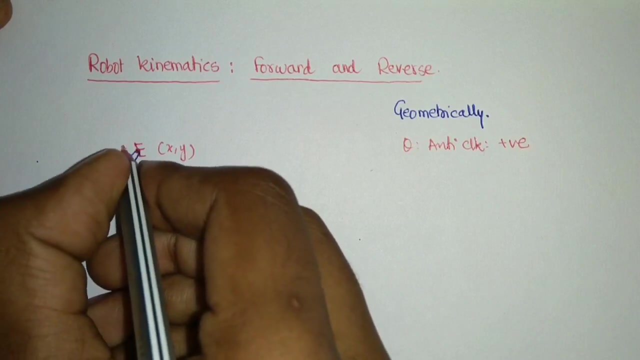 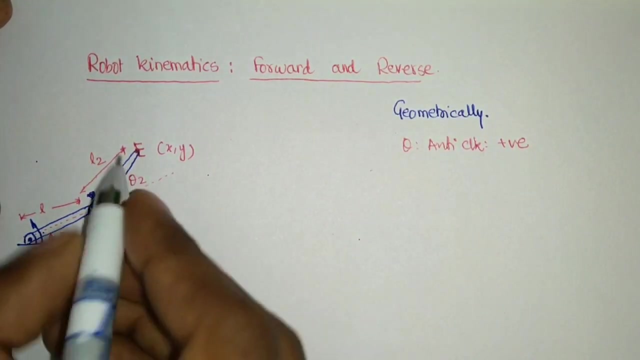 And the end effector's coordinates are x- y. Now, with the help of two links of length L1 and another link of length L2, and these two parameters, theta 1 and theta 2, I am able to finally have the position x- y and the overall position of this link is 5.. 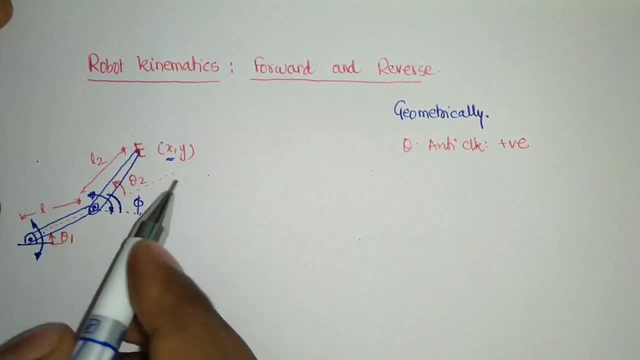 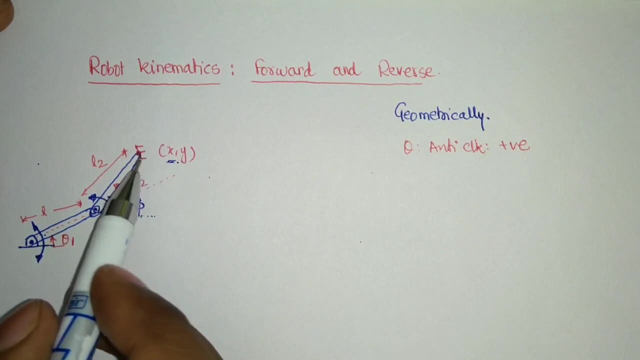 Okay, So 5 is the overall position with respect to the horizontal base. Okay, And theta 1 and theta 2 are individually associated with these links, L1 and L2 as well, And x- y is my final coordinate. 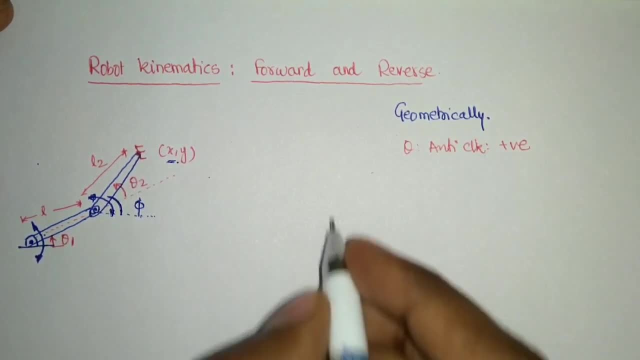 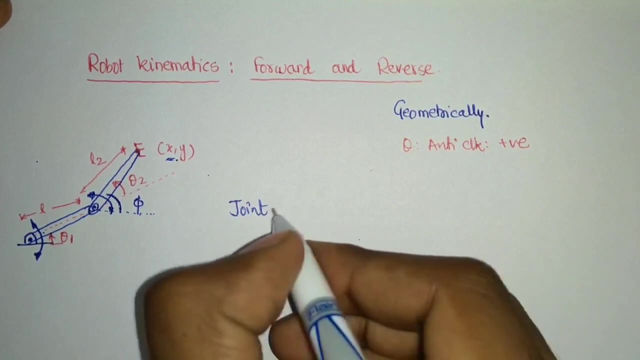 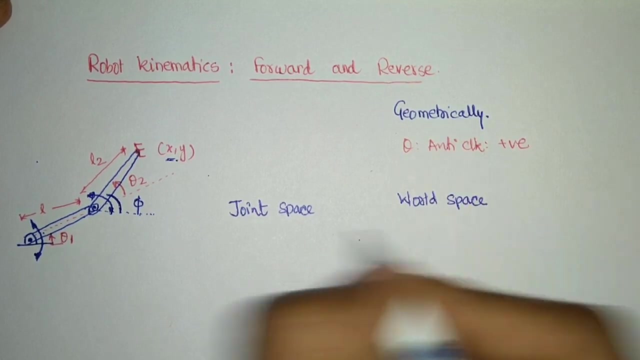 And the end effector. Now, when I say the forward or the reverse kinematics, I am basically going to have a conversion between the joint space and what we call as a world space. Okay, So what do I mean by joint space? 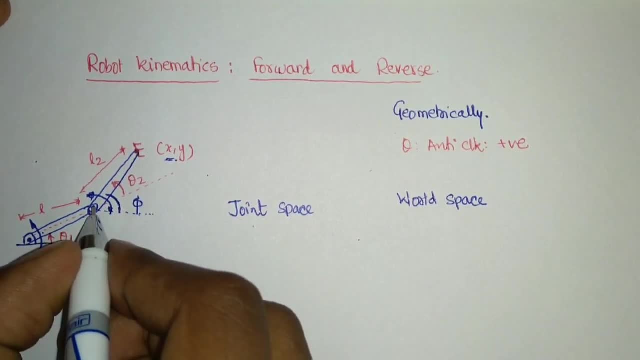 Joint space means the coordinate system attached to the joints, to individual joints. So theta 1 and theta 2 are basically the properties of my joint space. Okay, And when I say world space, world space means in terms of absolute coordinates. 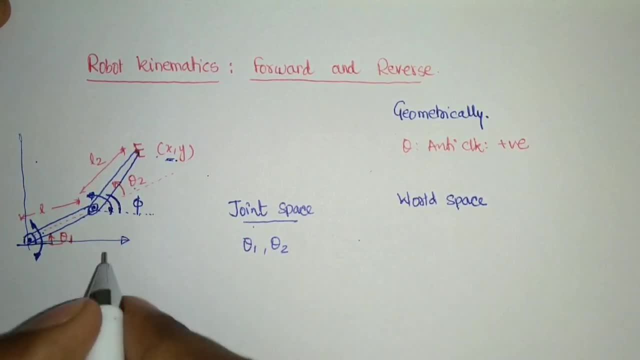 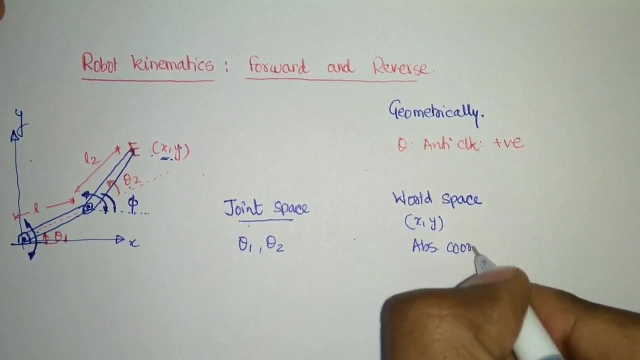 Okay. So if let's say this was my origin, Okay, x and y, two-dimensional only, we will take for now. So these x and y coordinates are giving me the world space or the absolute coordinates, I can say Absolute coordinates of end effector or the position of end effector. 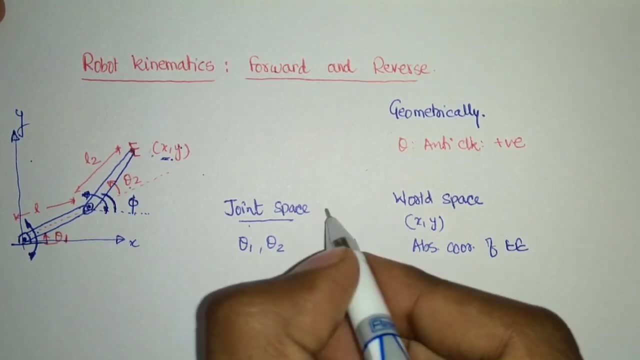 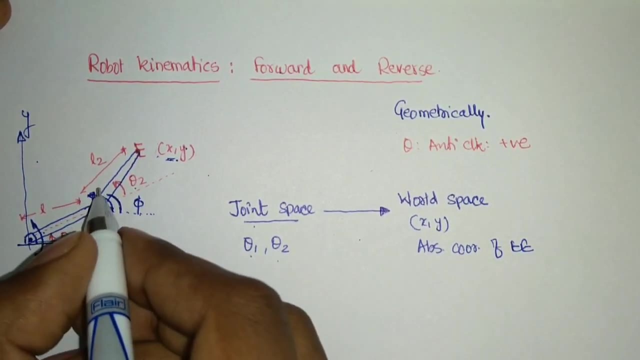 Now, whenever I want to know On the world space with the help of joint space, Okay, Meaning, I know theta 1 and theta 2.. Link lengths are, anyways, will be known always, And I want to calculate x, y and phi. 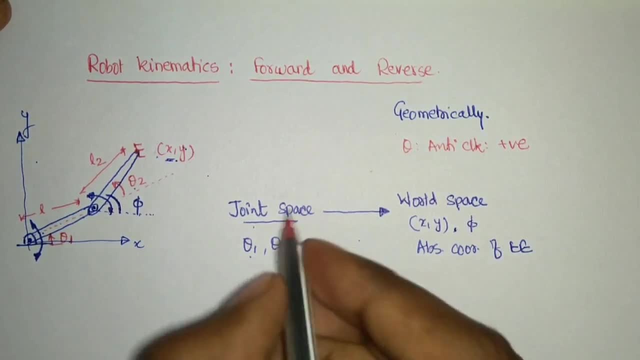 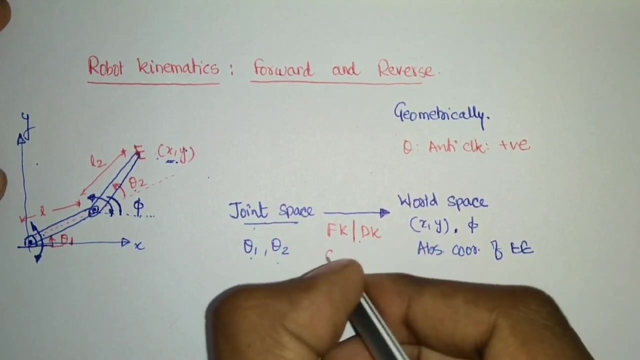 So how can I calculate that? So that system is known as forward kinematics. Okay, So going from joint space to the world space is known as forward kinematics, Or we also call it as direct kinematics. Okay, So this is obviously known as direct kinematics. 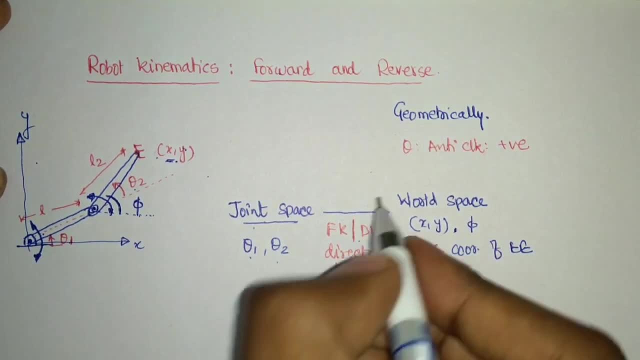 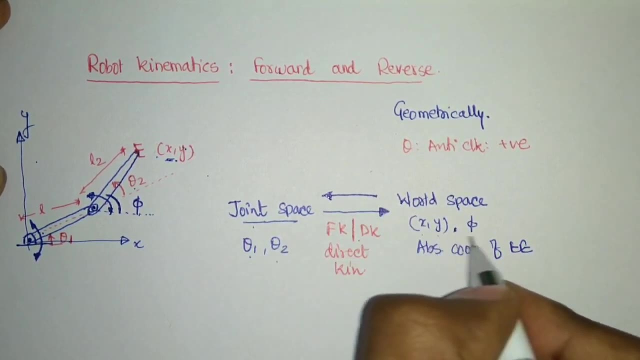 But when I go in reverse direction, reverse direction meaning when I go from world space to joint space. So this particular thing means I know x, y and I know phi And I want to know the value of theta 1 and theta 2 to orient my end effector in this position. 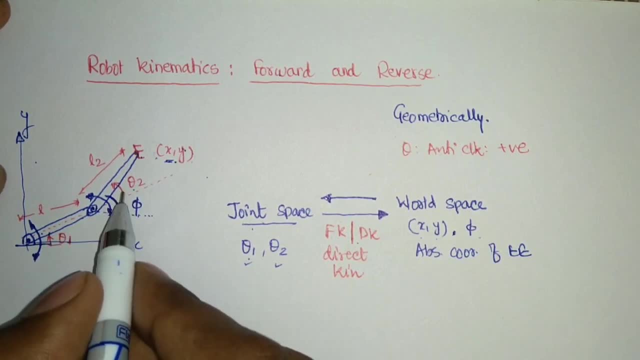 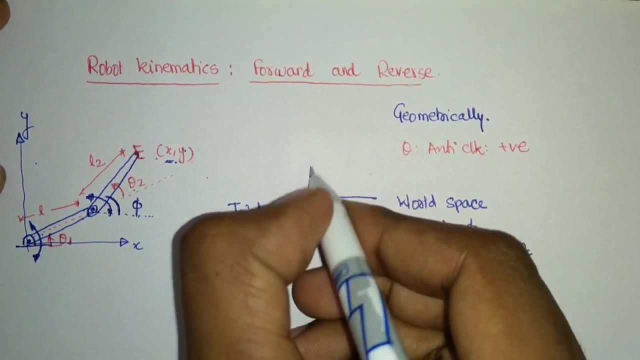 What should be the theta 1 and what should be theta 2 in order to give the command. Okay, So I know the world space, but I want to calculate the joint space. So that is my Reverse kinematics, Okay, 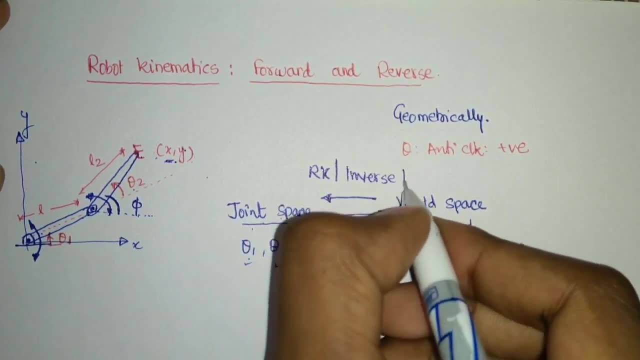 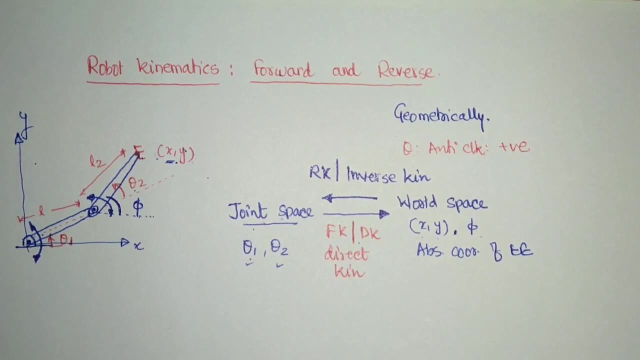 Or inverse kinematics. Okay, So that is the basic difference between the direct kinematics and reverse kinematics, Or forward kinematics and inverse kinematics. Okay, But why exactly do I want to do this transformation? Why can't I work with theta 1 and theta 2?? 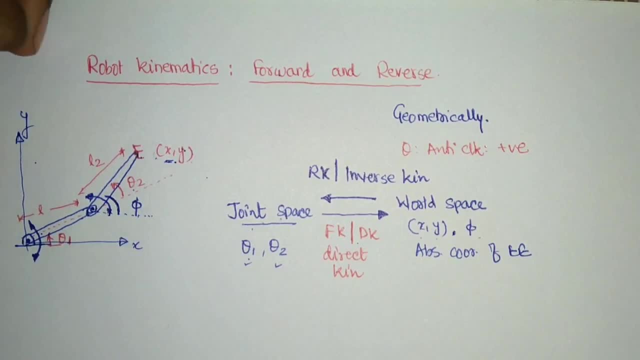 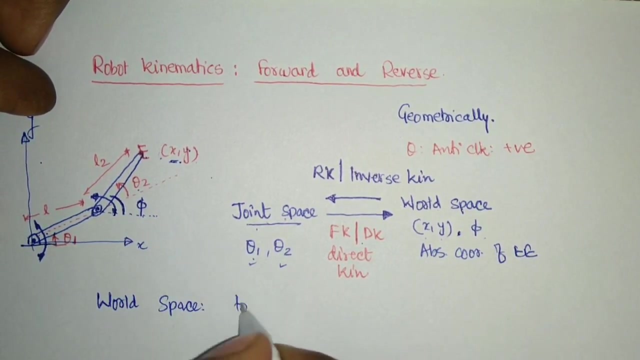 Why do I want these x and y? Okay. So the main purpose of having these x and y, or the world space, is to use the absolute coordinate system, Okay, Okay, And to communicate with the external world. So the world space is basically to communicate with external world. 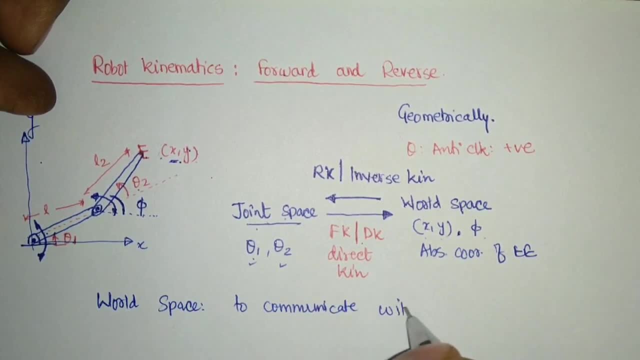 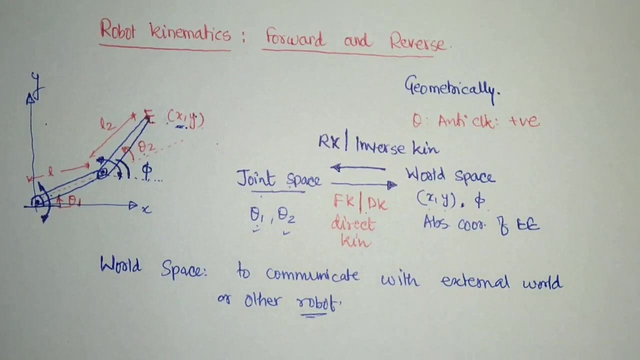 To communicate with external world or robots. Okay, So, whatever system that we are having in our machinery or in our plant productions, of anywhere, we need this robot to work. We need this robot to work. We need this robot to work. We need this robot to be able to communicate with other devices, other robots. 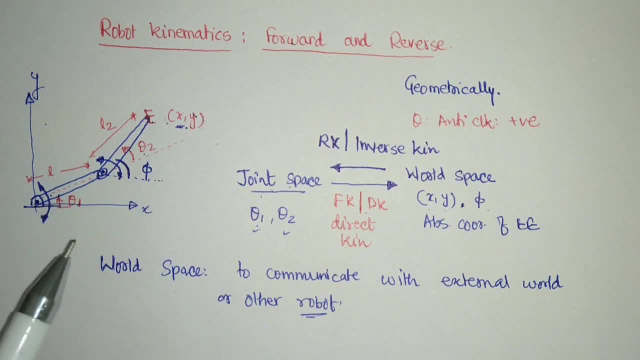 Okay, In order to do that, we need to give the position with respect to the absolute coordinates, And that will be done with the help of a forward kinematics. Okay Now, in order to carry out the forward kinematics, the two approaches that are very common and 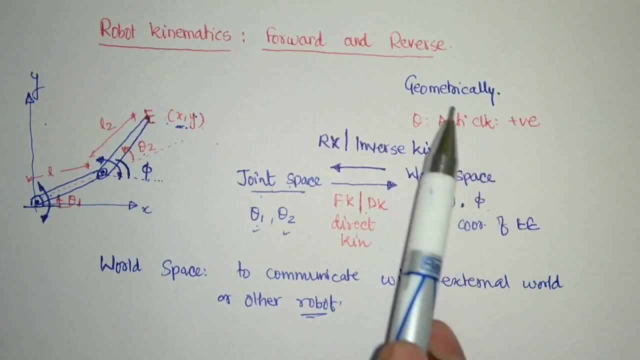 very useful. One is the geometrical approach, which we are going to discuss here. The geometrical approach we will be taking up for 3 degrees of freedom as well as 2 degrees of freedom, Okay. And another one is TH- forward kinematics. 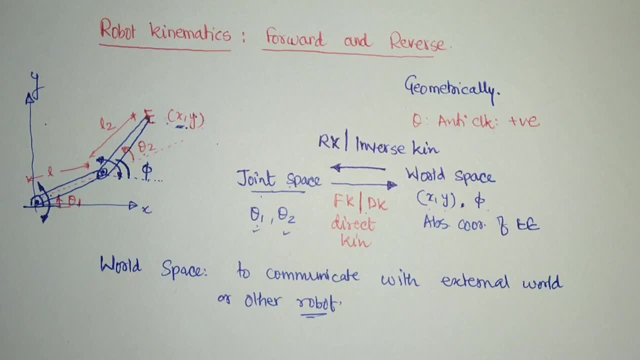 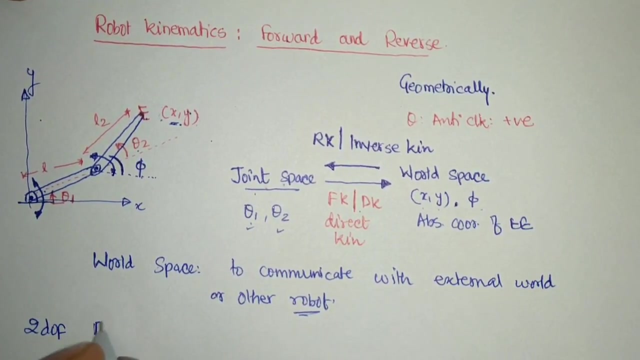 That is that we will take up later, because it's a bit complex and lengthy also, but important from the main point of view. Okay, So now let's do this. 2 degree of freedom: direct kinematics analysis. Okay So, 2 degree of freedom: forward kinematics. 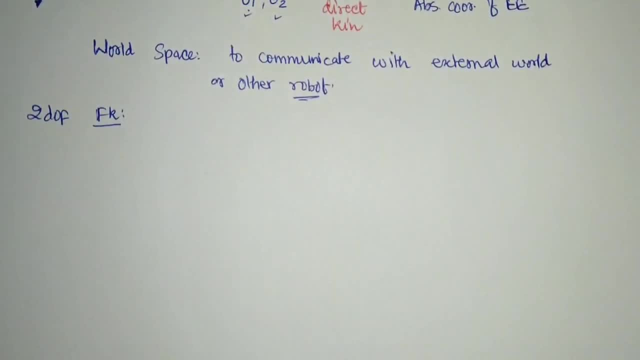 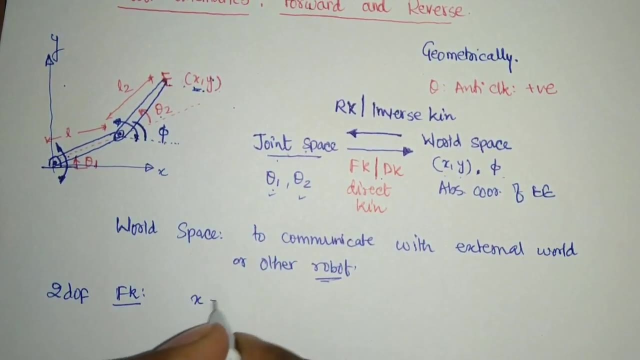 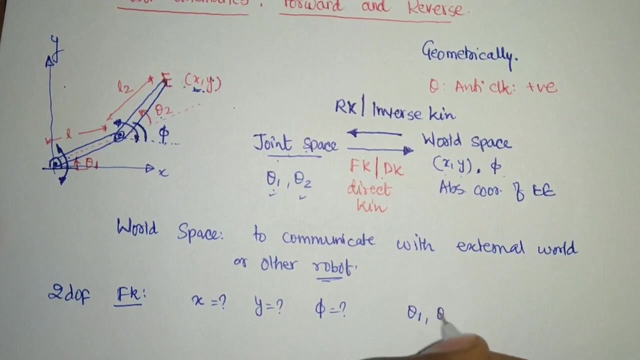 Okay. So when I say or when I do a forward kinematic analysis for this one, So what I basically want to know, the value of x and y and phi in terms of x, So what I basically want to know, the value of x and y and phi in terms of x- is already. 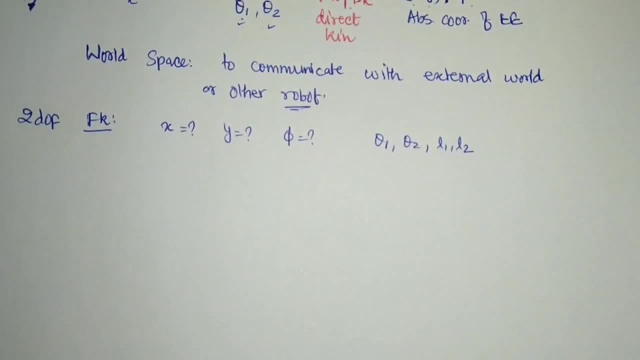 given as x. So what I basically want to know: the value of x and y and phi in terms of x. Let me just have a look over here. So let's see what I am given as, and y and phi here. 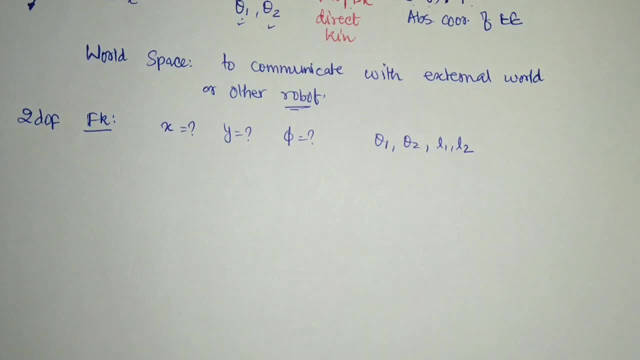 So now I am given here x, x, y and phi, And I am already given theta 1, theta 2, and my link lengths. So link lengths will always be known to me. Okay, There is no way that I don't know the link lengths actually. 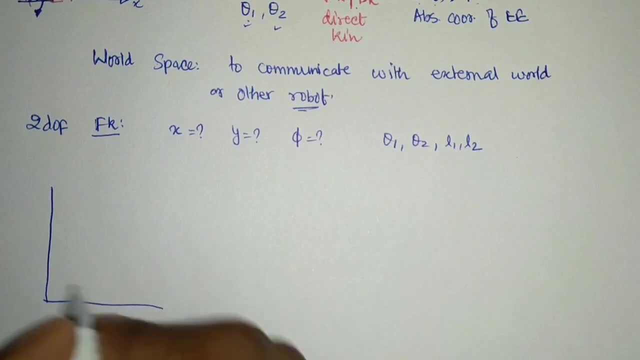 In order to do that here, I will say: and this is my system, right, This is theta 1. and I will say that I am given this theta 5.. This is theta 5.. and this is my system, right. this is theta 1,, this is theta 2, and these are x- y coordinates. 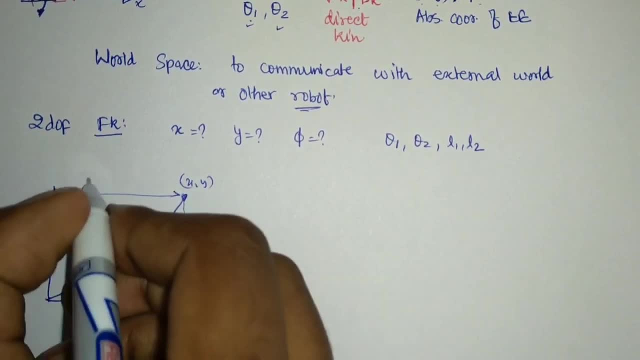 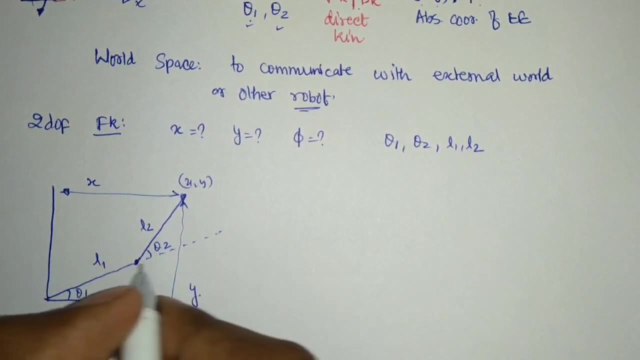 so this length is basically x length and this length is basically y length. okay, and l1, l2, I already know if I can give them in terms of this whole length can be divided, or I can say that it can be subdivided into two parts, this plus this, okay. similarly, 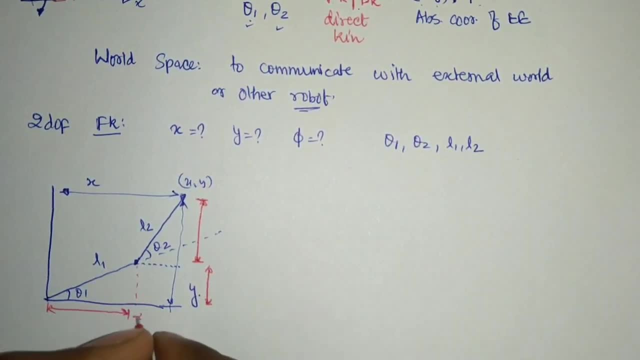 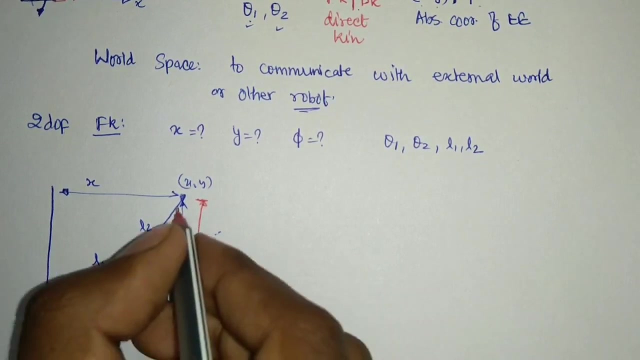 the horizontal length can be divided into two parts: this and this, okay, and as we can see that, if this is l1, this length will be l1 cos theta 1, okay, and this length will be l1 sin theta 1, right, this vertical length, this length, this length is going to be l2 into cos of this. 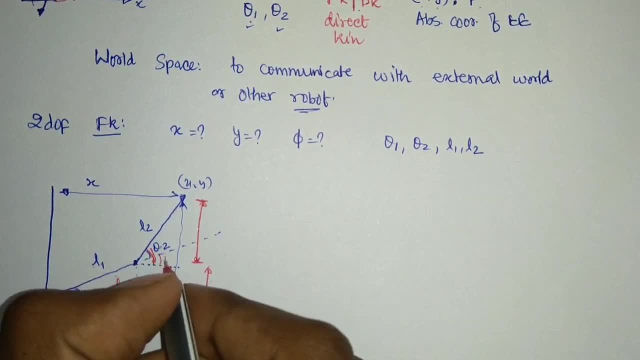 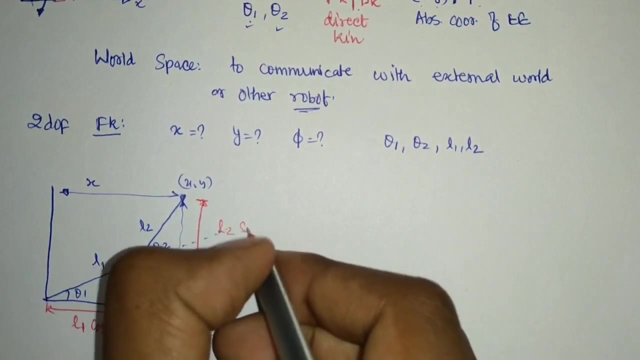 whole angle and that whole angle is theta 2 plus theta 1,. okay, because this is theta 1,. right? so that is going to be l2 cos, theta 1 plus theta 2, and this is going to be l2 sin of theta 1 plus theta 2,. okay, and whenever. 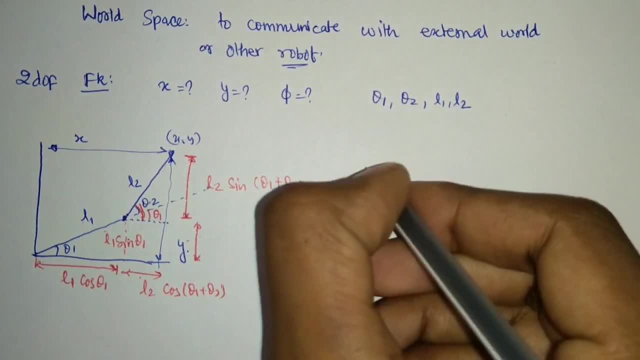 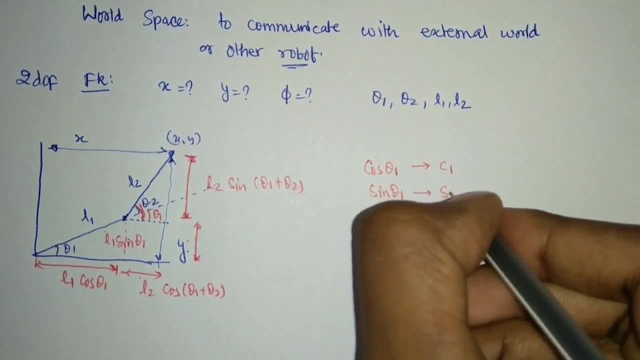 we are doing a kinematic analysis in a robot. we don't write as cos theta 1 or sin theta 1, we will simply say c1, and this will, so that will directly give us cos theta 1, this will. 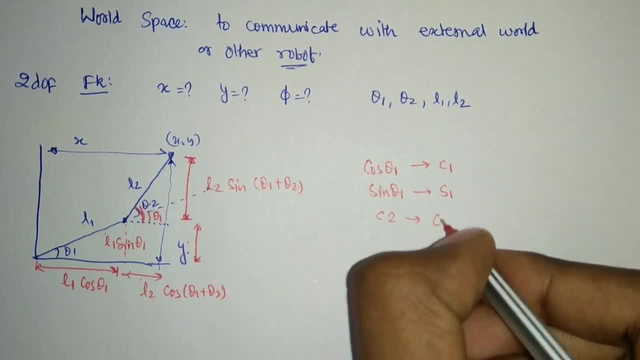 simply sin theta 1.. Similarly, c2, that means cos of theta 2,. okay, c12 will mean cos of theta 1 plus theta 2,. okay, it is not cos theta 1 into cos theta 2,, it is cos of theta 1 plus theta 2,. similarly, 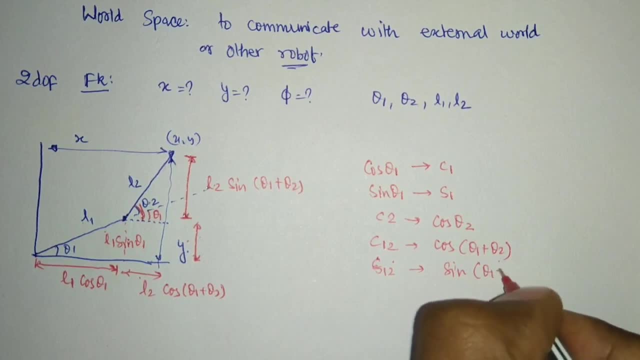 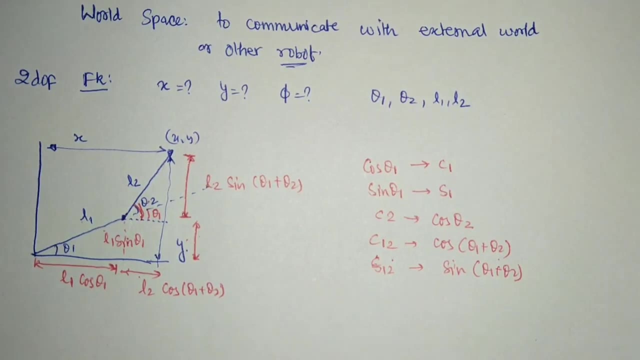 s12: sin theta 1 plus sin theta 2, sin theta 1 plus 2, okay, that sort of analysis, that sort of notation we use here. okay, now I can very easily say that my x value is equal to this plus this right. 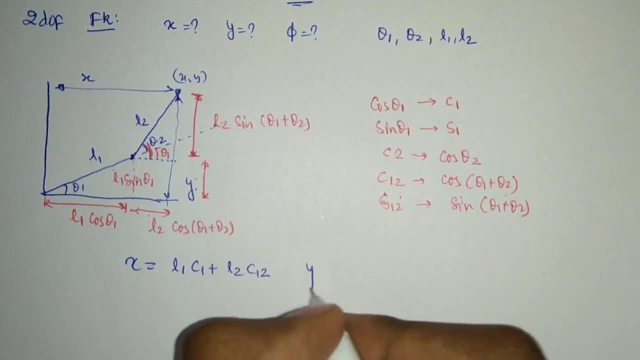 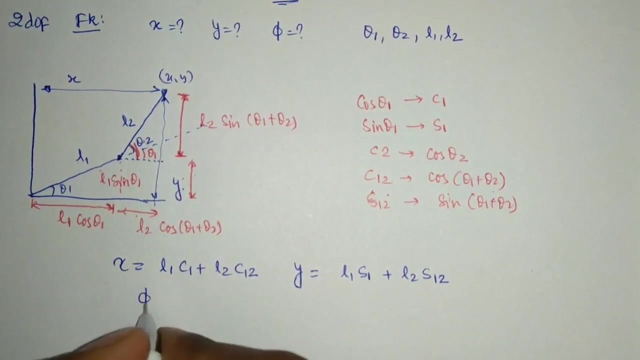 l1 c1 plus l2 c12, and my y value is equal to l1 sin theta 1 plus l2 sin theta 1 theta 2, right. so that is my forward kinematics right and phi is equal to theta 1 plus theta. 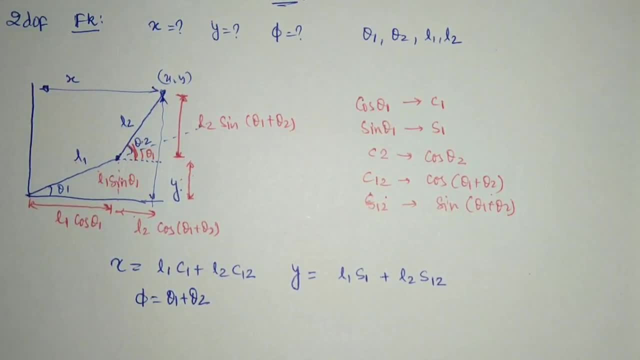 2, you know, if there is a question regarding forward kinematics, that is what we need to do, only this much. okay now, in this itself, if I want to carry out the inverse kinematics or the reverse kinematics, so what will that mean? so that is a forward kinematic. 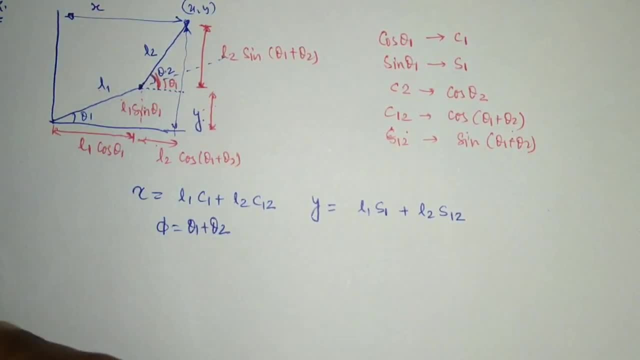 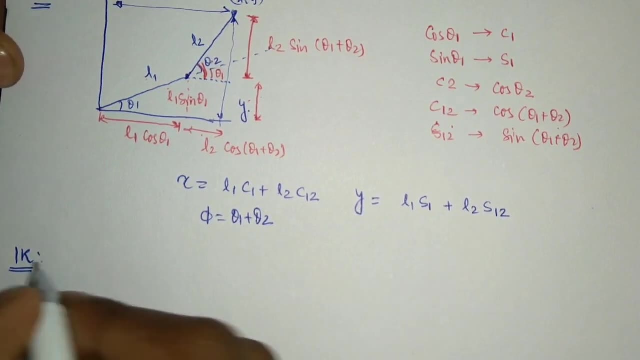 analysis. okay, now I want to do the inverse kinematics analysis. sorry, I want to do the inverse kinematic analysis. in inverse kinematic analysis, I already know x and y are given to me and phi is given to me. what I want to know, theta 1 and theta 2, always link. 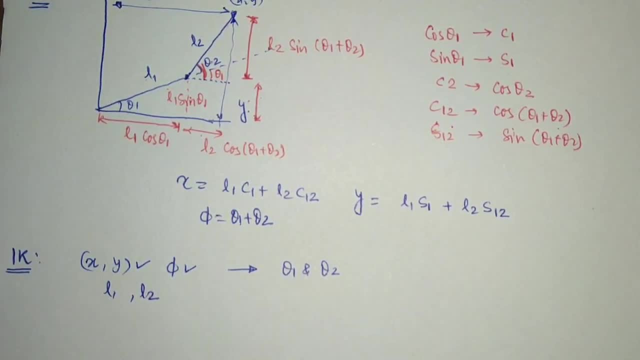 lengths will be given and known okay. So there is no doubt about, or there is no question of knowing the link lengths right now. how do I do that? so one thing that I can do is I will simply square them both. 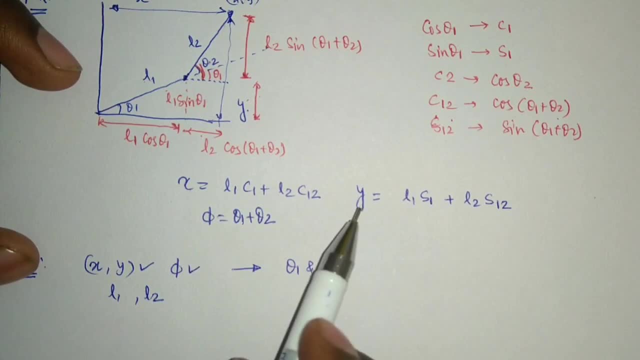 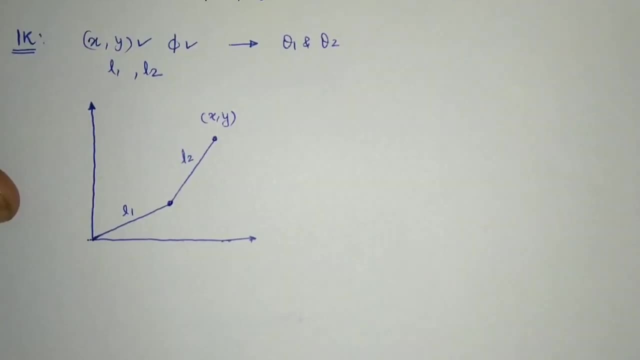 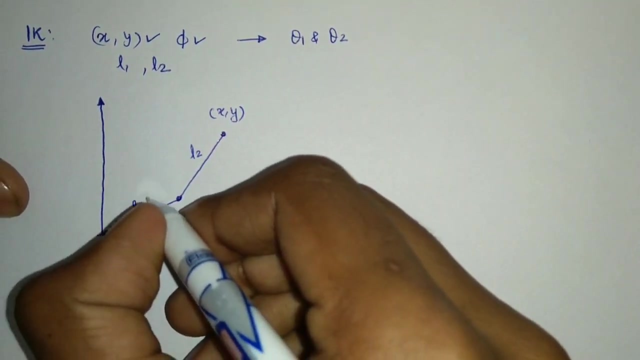 sides x square and y square. okay, both sides square, both sides added up, and then I can simply solve it. okay, another okay. so, as I said, we are going to square the x and y and add that together. okay, so x square plus y square can directly be given by this. 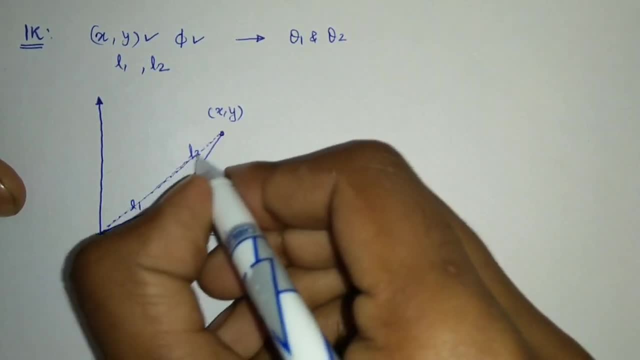 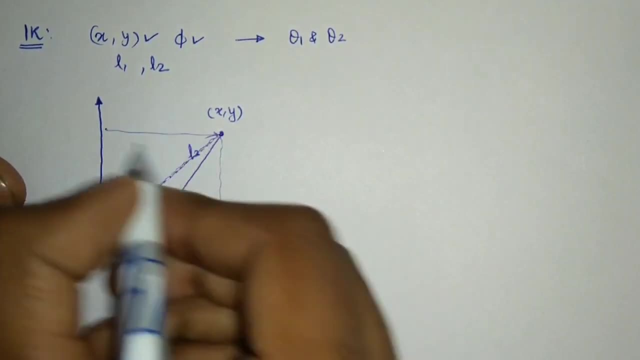 length, okay, or the square of x and y, and then I can simply add it up: okay, and then this particular length: right, that will give me x square and y square, because this height is y and this length is x, right, so simple hypo, this right triangle theorem, right. 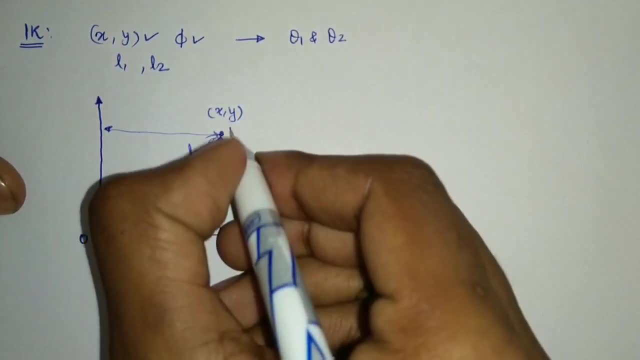 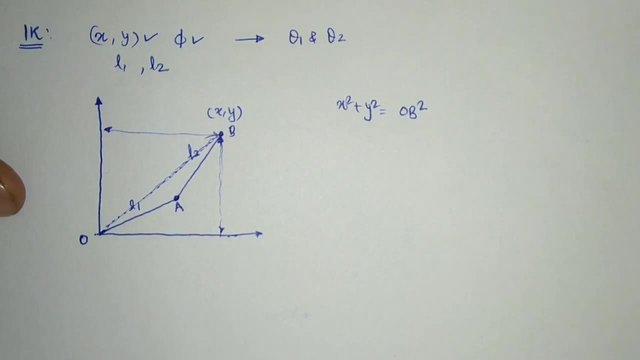 so this length will be my, or I can say o, a and b. so ov x square plus y square is basically nothing but ov square, right, but I can write that in other terms also or in other ways also. 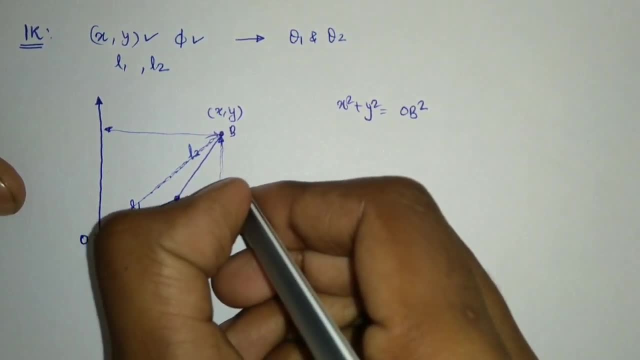 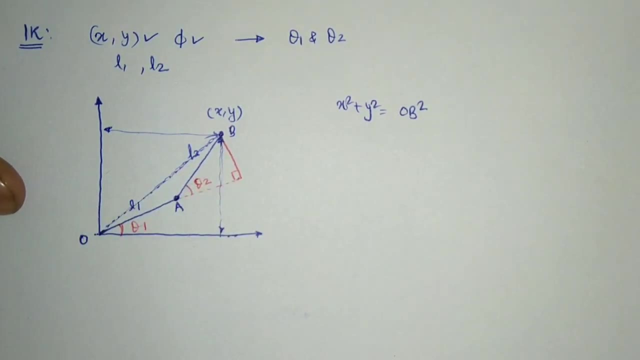 I want to know these angles. Okay, So I want to know these angles, theta 1 and I wish to know theta 2, this is my theta 2 over here. right, these two angles I want to know so I can say that square, if this point. 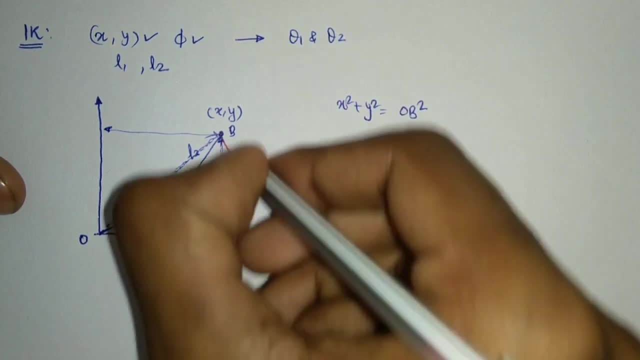 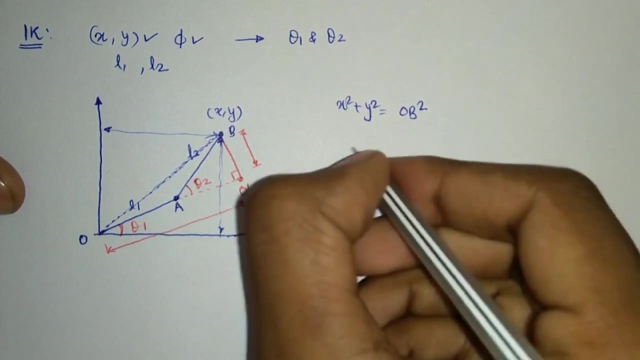 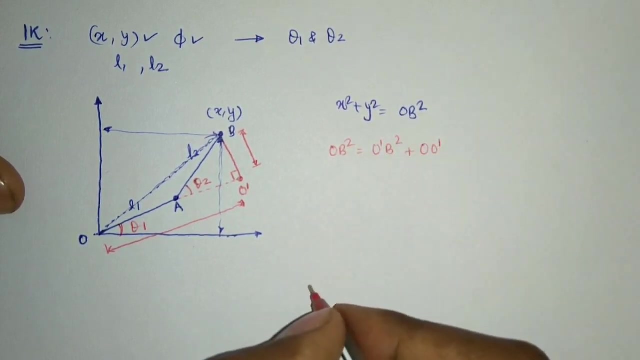 is, let us say, o dash, then square of this length plus square of this length right. so same ov square is equal to o dash b square plus o. O dash is square right and o dash b. I already know that o dash b is nothing but l2 sin theta. 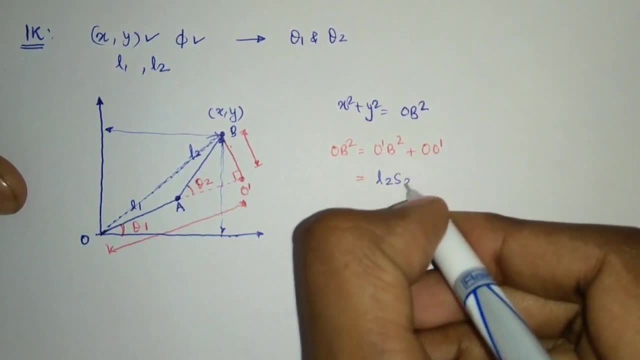 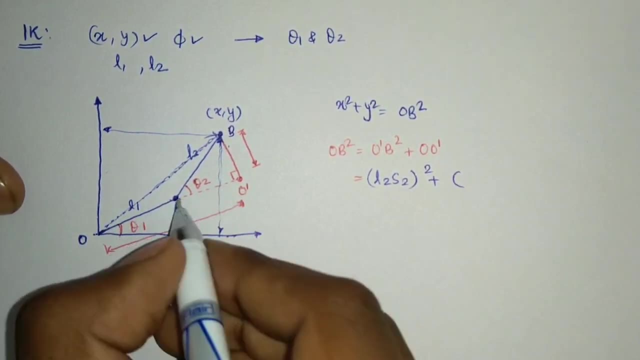 right l2 sin theta. so l2 sin theta 2 square plus o o dash. o o dash means this length, and this length is equal to l1 plus l2 cos theta right, so l1 plus l2 cos theta square. 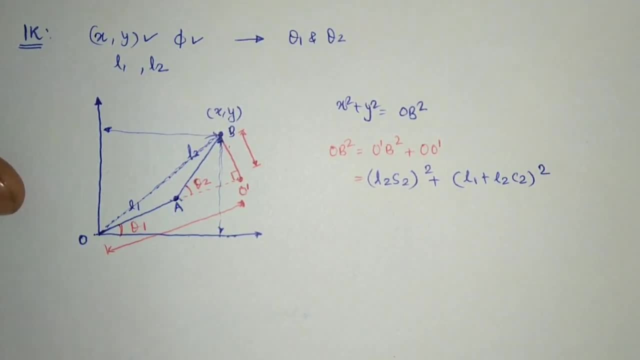 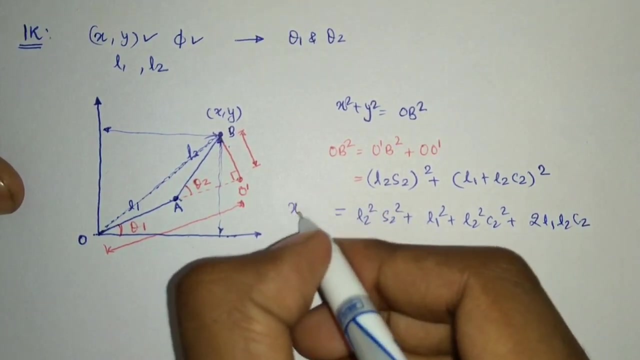 cos theta 2 square right now I can simply expand it. okay, And expansion will give me l2 square, s2 square plus a square plus b square plus 2abc2, right, that is my equal to x square plus y square, and this l2 is 2 square and l2c2 square that. 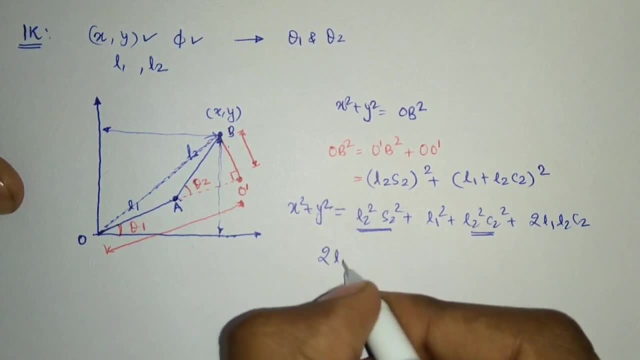 is giving me l square simple right. So the only term that I am remaining with is 2l1l2c2 is equal to nothing but x square plus y square minus l1 square, minus l2 square. Okay, and c2, or my cos of theta, 2, is equal to x square plus y square minus l1 square. 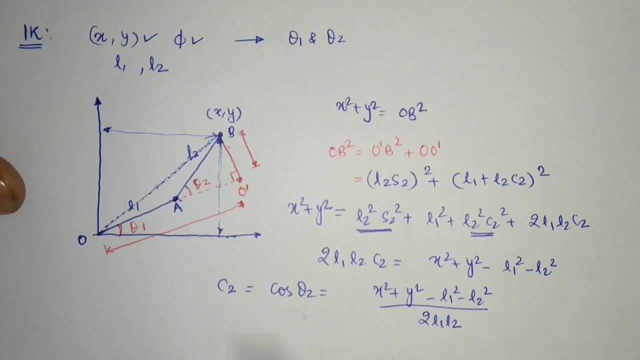 minus l2 square divided by 2l1l2, and that is the final answer that I will be having for cos theta 2,. okay, Now I simply can take a cos inverse here and I can get the theta 2 value from here. 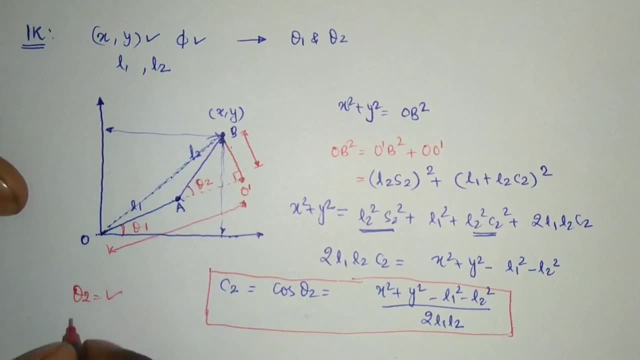 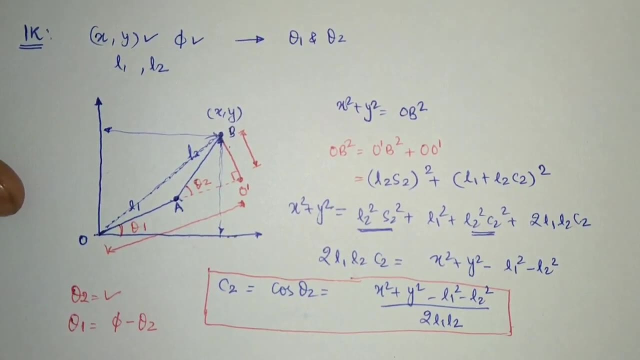 okay, theta 2 value I can get Similarly when I know phi, So theta 1.. So theta 2 will be equal to phi minus theta 2, and that will give me my final answer. Now there is a catch here, and the catch is that inverse kinematics may not have a unique 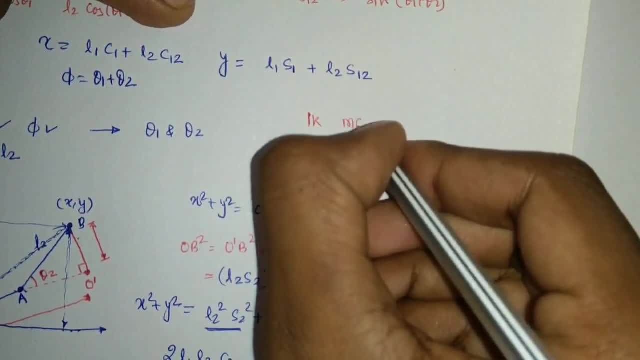 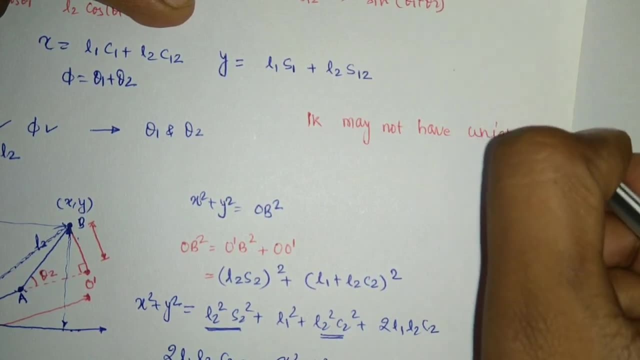 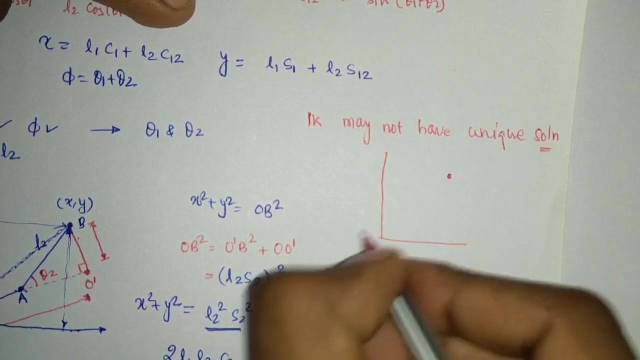 solution. okay, So inverse kinematics may not have a unique solution. What do we mean by that? That it may not have a unique solution? is that the only thing that we needed was this position at the end? right, Right, Right. 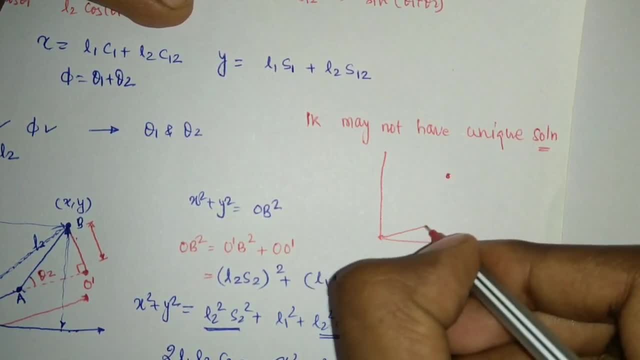 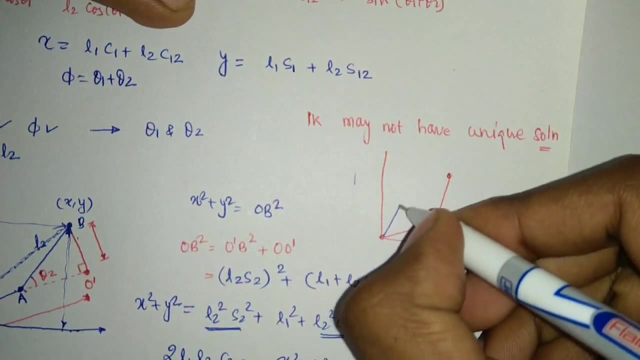 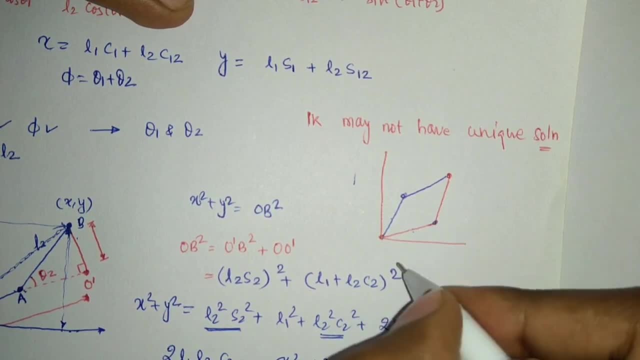 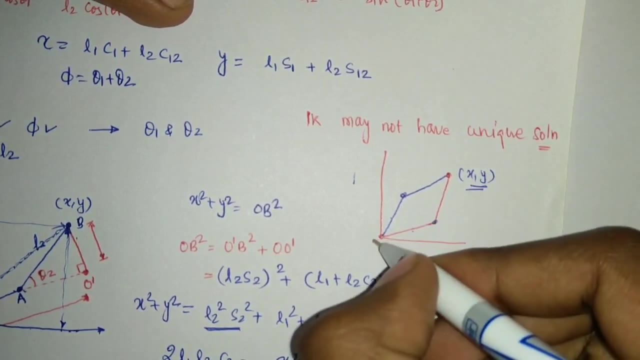 Both link lengths are same: L1 and L2.. But two configurations are possible. here Means I will be getting two solutions to get this: x and y. That is why usually we define whenever we are programming we will define that we want an under solution or an above solution. 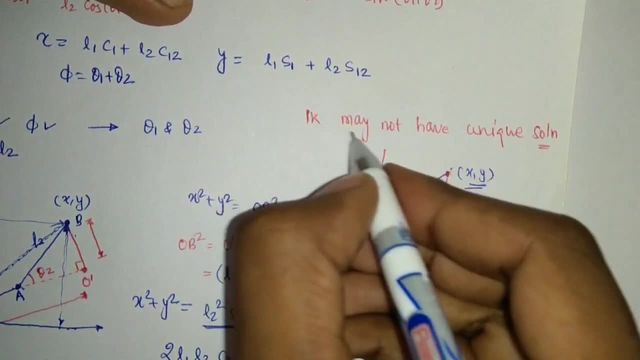 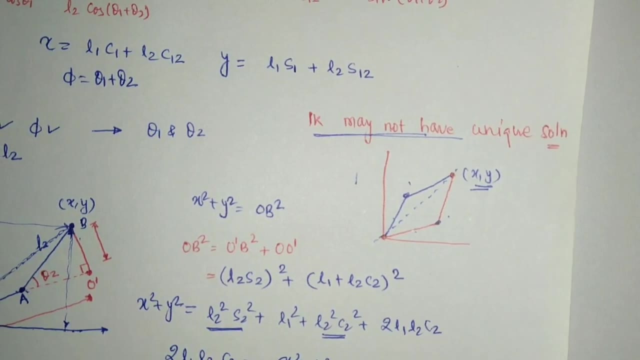 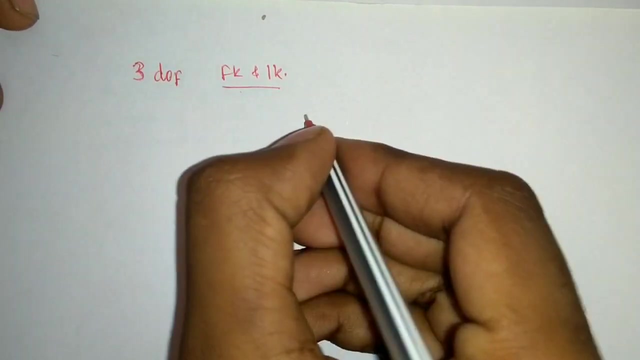 Usually that has to be under solution given. okay. so this may also be asked that inverse kinematics have unique solution or not. so we can write that okay. so that is all the forward and reverse kinematics of a two degrees of freedom, three degrees of freedom, the forward kinematics as well as inverse kinematics. 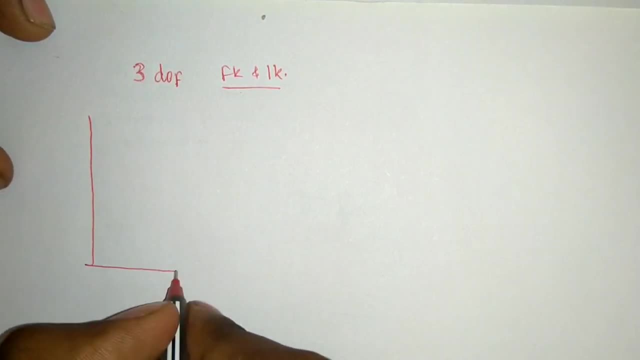 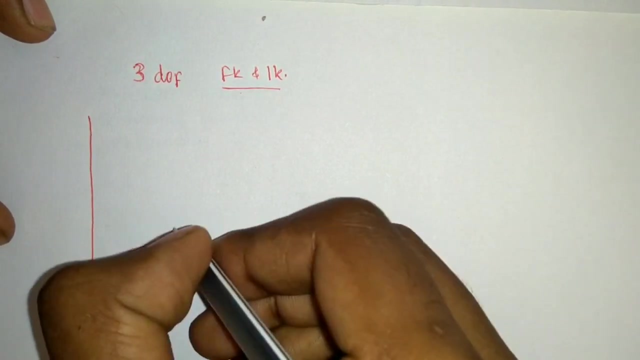 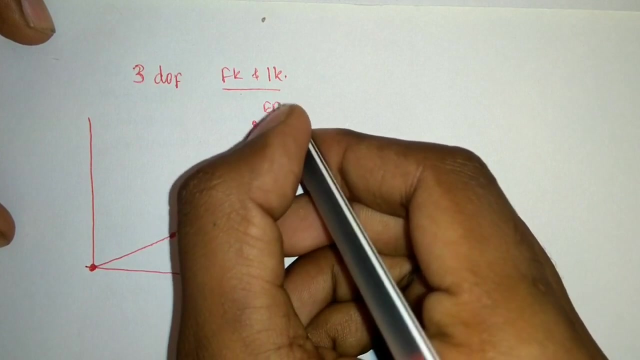 with all rotary joints, okay. so basically the problem that we are having here is there is a rotary joint joint one- okay, there is a link over here. then there is another link- rotary joint- and then there is a thread link. this is my and effector here, okay, and all the things. 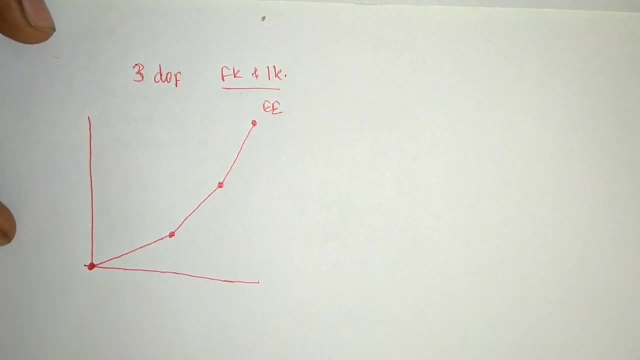 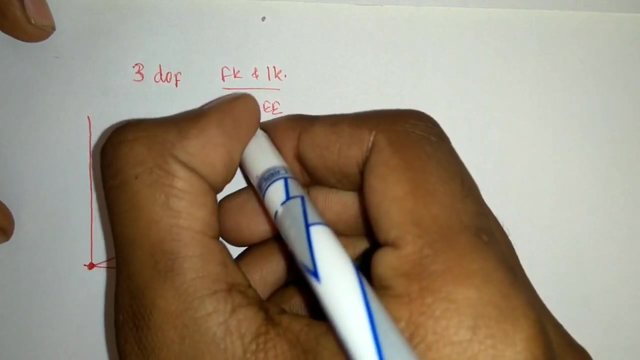 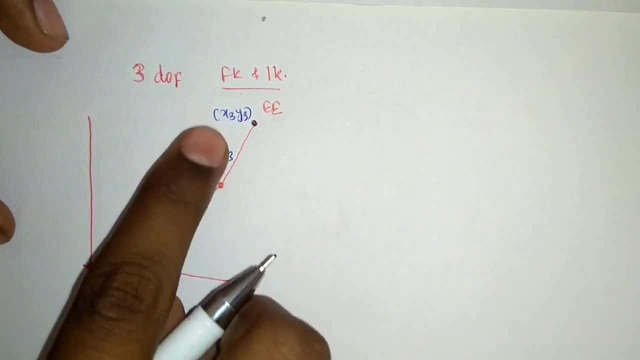 that i'm having over here the coordinates. let's assume this is x1, y1, this is x2, y2 and this is x3, y3. link lengths are l1, l2 and l3. finally, i want to calculate my x3 and y3 given. 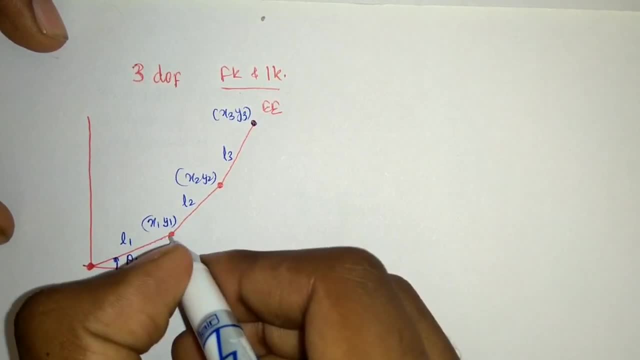 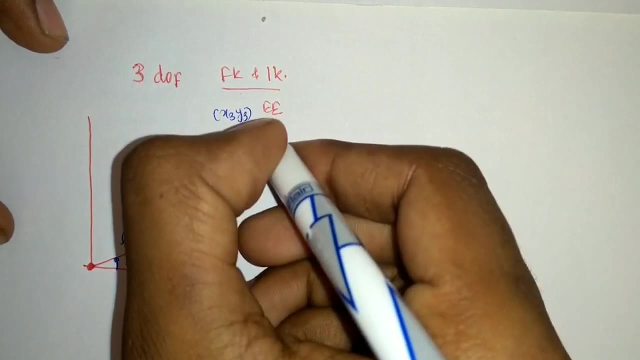 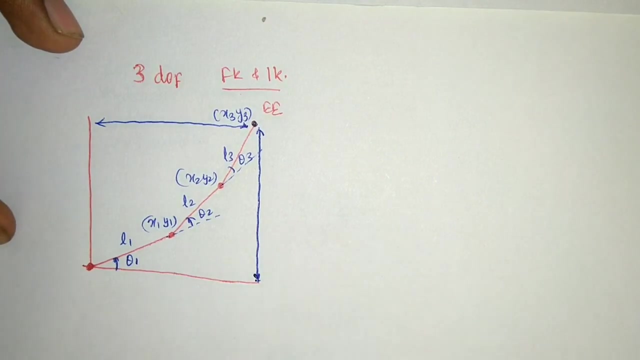 that the joint parameters in a theta one, second theta 2 and third theta 3. I already have them, so I need to calculate this length, which is x3, and this length, which is y3. ok, so, in order to do the forward kinematics, I can do it very. 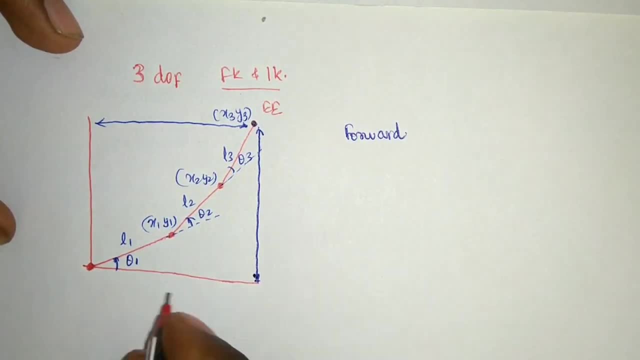 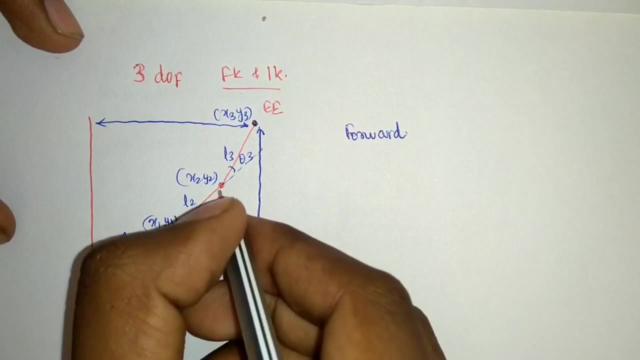 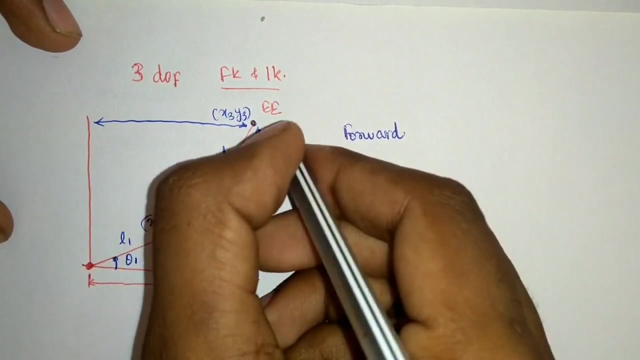 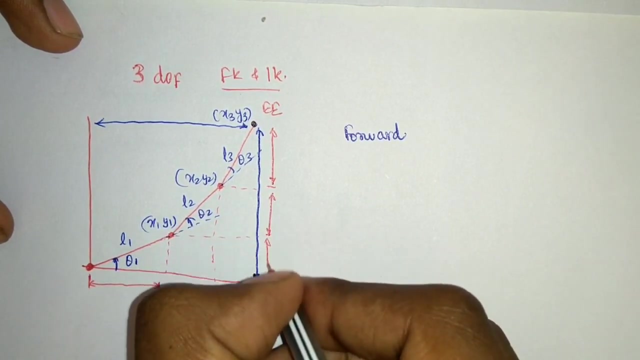 simply using the geometric relationships here: ok. so x value means this total length can be divided into three lengths here. ok. so this length plus this length plus this one- ok. similarly, y can also be divided into three parts plus this one. ok, so all these lengths we can write. 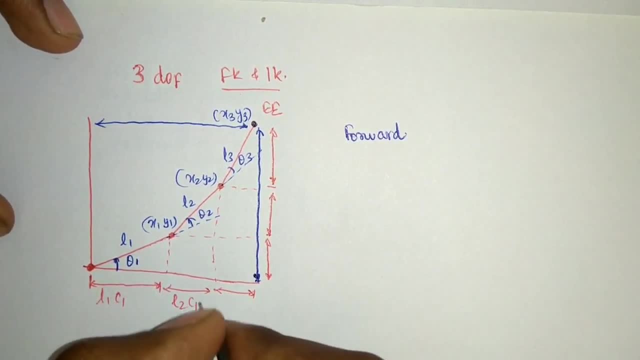 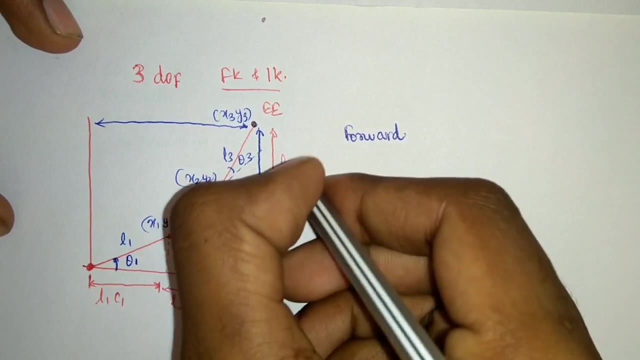 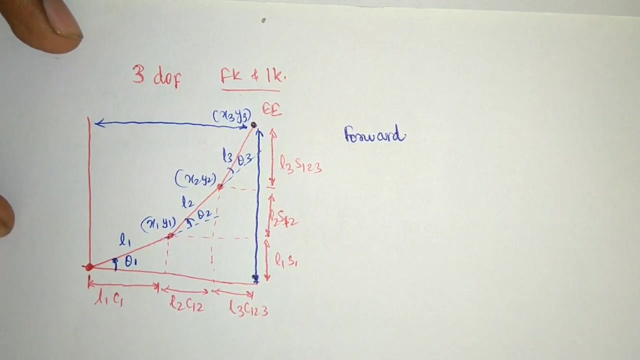 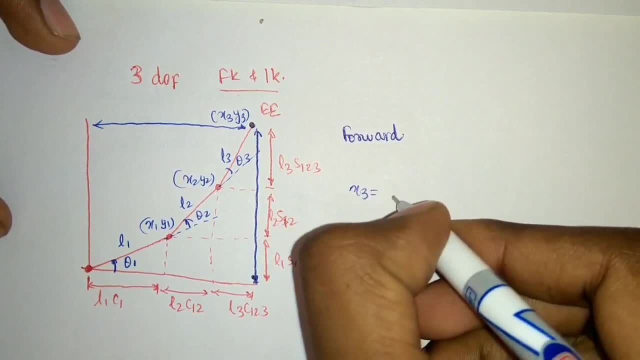 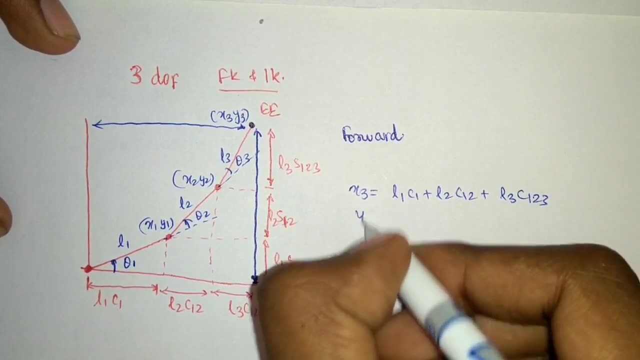 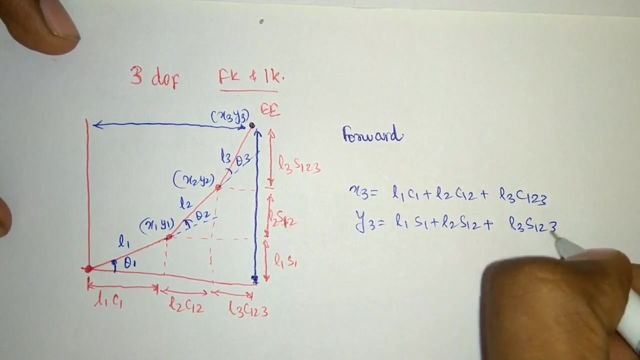 transformations. ok, so my x3 will be equal to l1 c1 plus l2 c12 plus l3 c123 and my y3 will be equal to l1 s1 plus l2 s12 plus l3 s123. right, that is how I can do the forward. 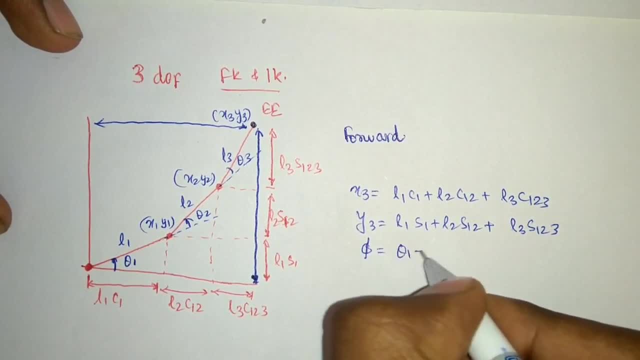 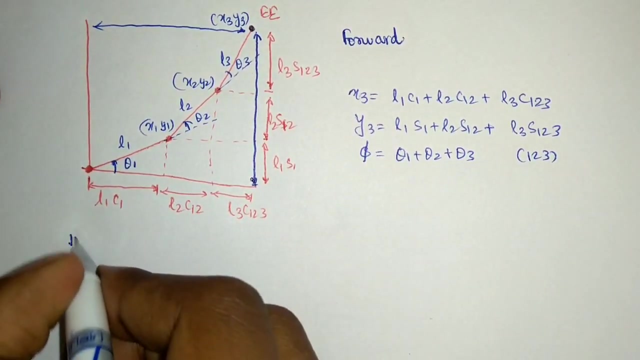 kinematics. One more thing I can calculate is: phi is equal to theta1 plus theta2 plus theta3, or simply 1 to 3, right, that also I can calculate. so that is all about the forward kinematics. Now, if I look at the inverse kinematics of this same system here: ok, so in order to do 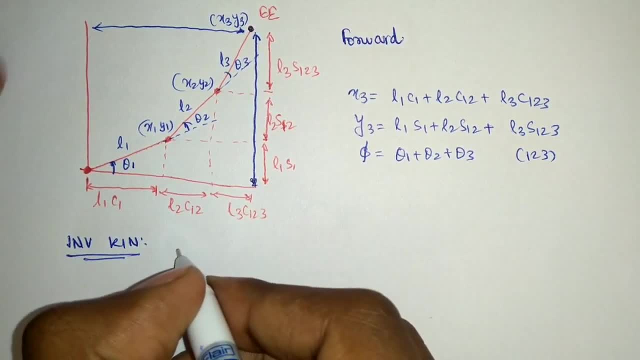 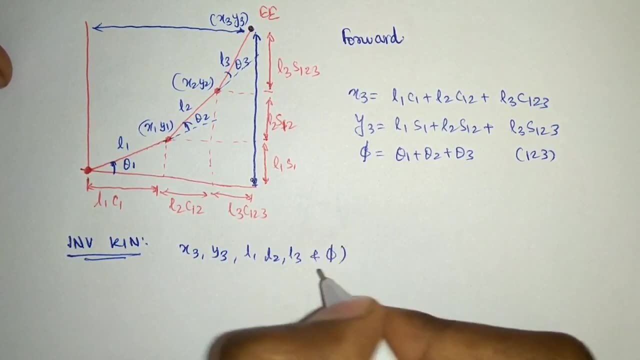 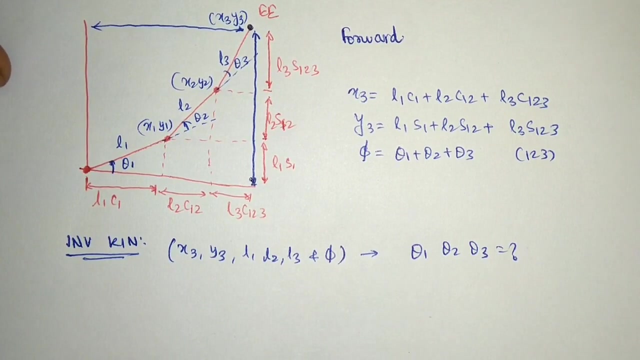 the inverse kinematics here means I will be given x3, y3, l1, l2, l3 and phi- all these values- and I need to calculate theta1, theta2 and theta3 over here. ok, what will be those values? so when I try to solve this equation, the first thing is I try to write x2, y2 in terms of: 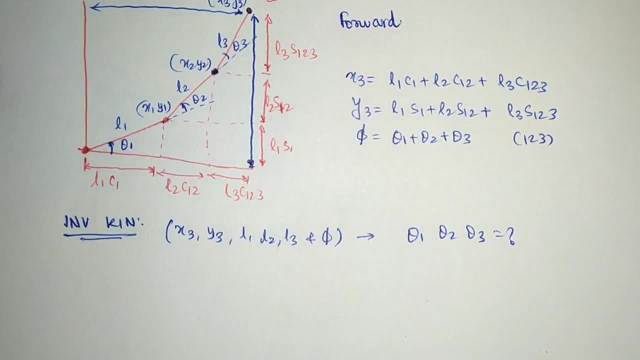 x3, y3 and in terms of lengths, or the length lengths. ok, so I can say the very first equation is that x2 is equal to x3 minus l3 cos of phi. ok, because phi is nothing but theta1 plus theta2 plus theta3. ok, 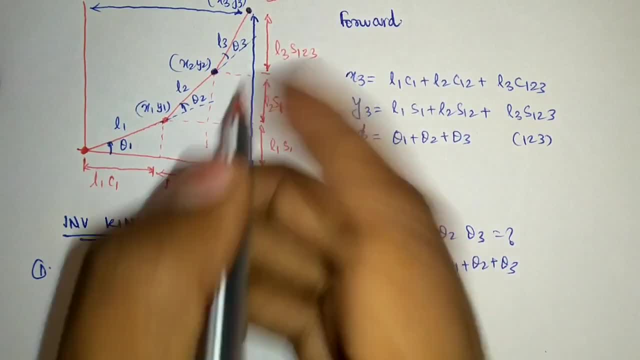 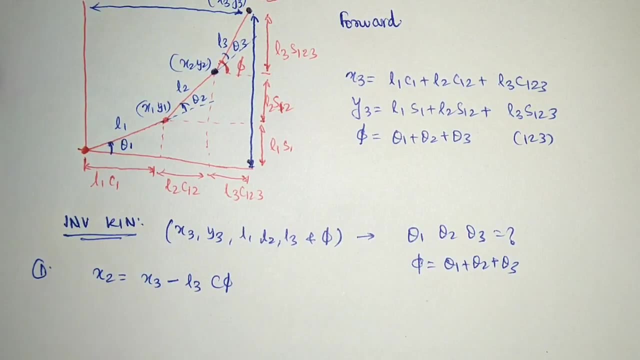 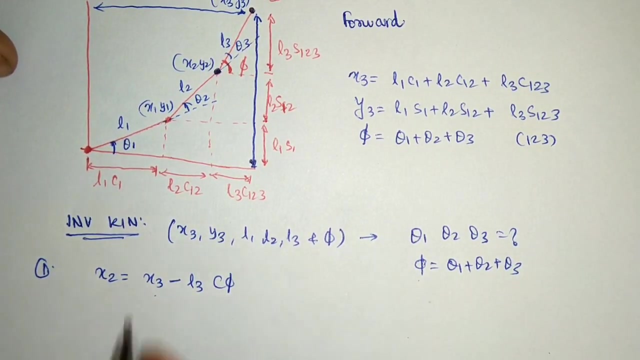 Ok, What phi is over this angle? this total angle is phi. ok, the total angle we are having here is phi value. so phi is equal to theta1 plus theta2 plus theta3. x2 value can be written in terms of x3, because x3 we already know. that is why we are writing it in this way. 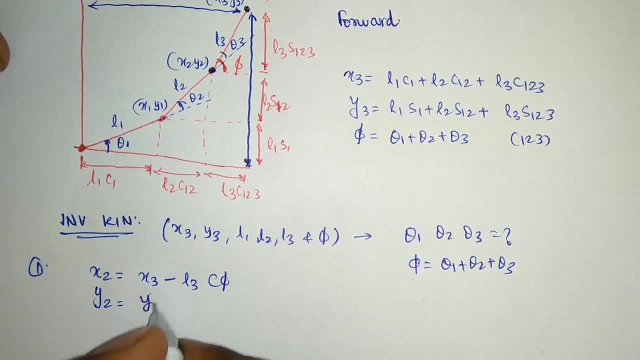 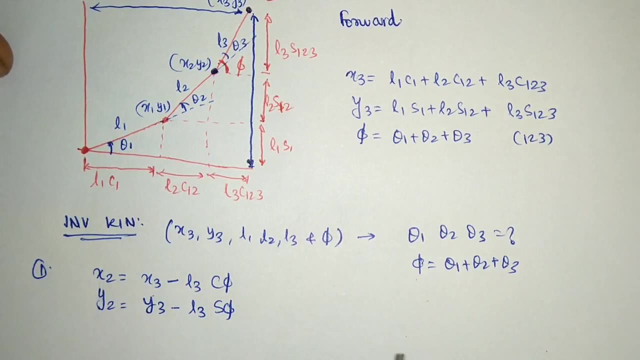 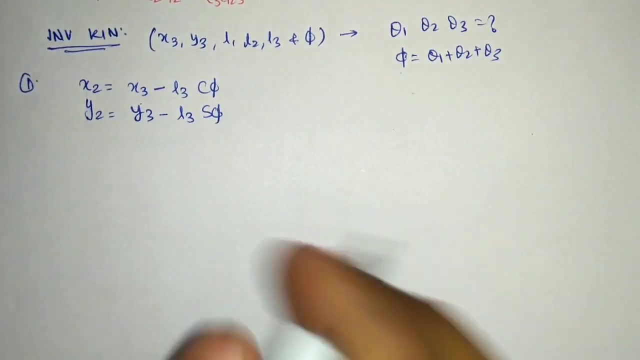 and y2 will be equal to y3 minus l3 sin phi. ok, Now, using these two equations, we can now apply the same analysis as we did for y2 and y3, as we did for 2 degrees of freedom, and that will give me simply this desired relationship. 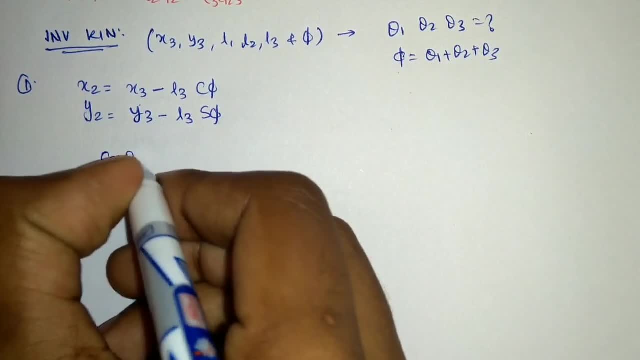 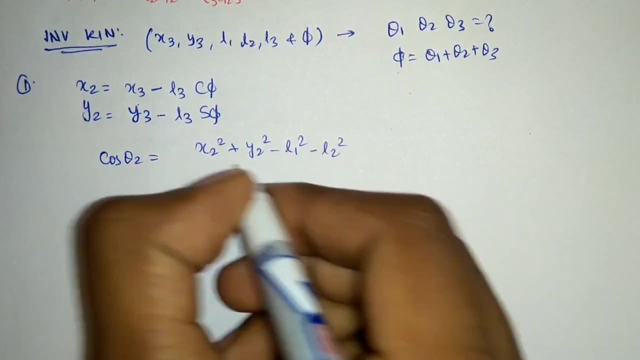 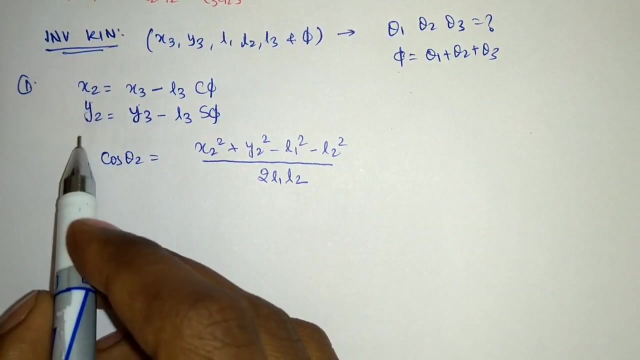 which is cos of theta2 is equal to x2 square plus y2 square, minus l1 square minus l2 square divided by 2 l1 l2. ok, because I already know x2 value and y2 value, I can now apply this one, ok. 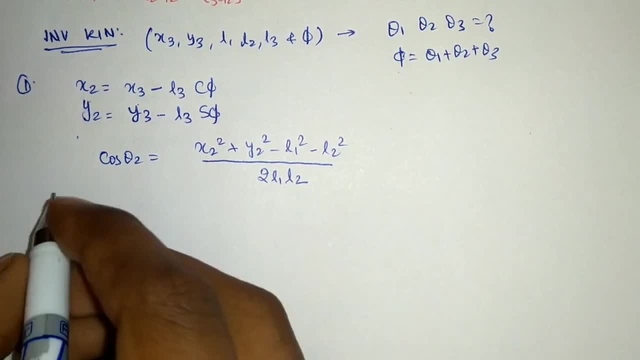 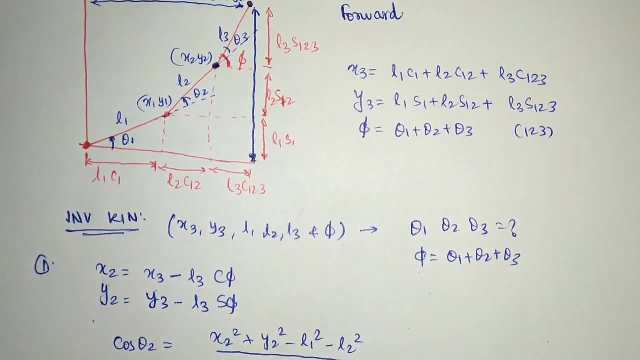 Ok. Ok, So I can say x2 and y2 will be that I can say: x2 is equal to l1 c1 plus l2 c1- 2. right x2 value is equal to l1 c1 plus l2 c1- 2. similarly, y2 is equal to l1 s1 plus l2 s1- 2. ok. 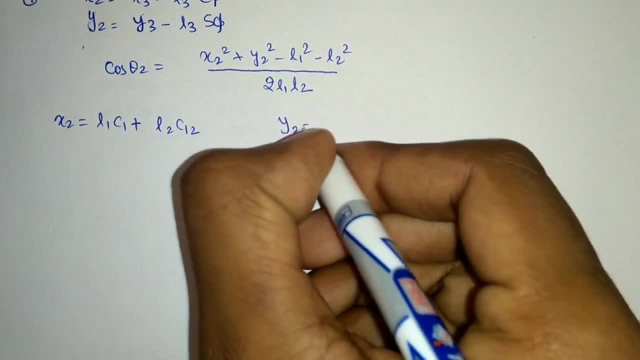 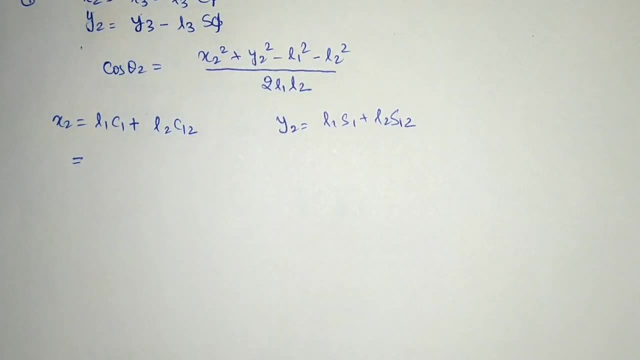 So these two equations I am going to use here, y2 is equal to l1- s1 plus l2, s1- 2. now expanding this one it will give me I will finally get. so I will apply the formula of c1- 2 here. I. 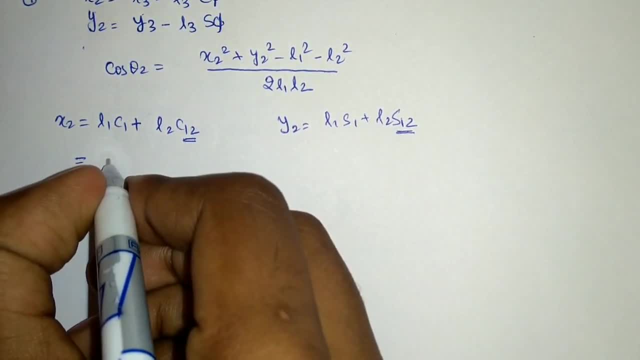 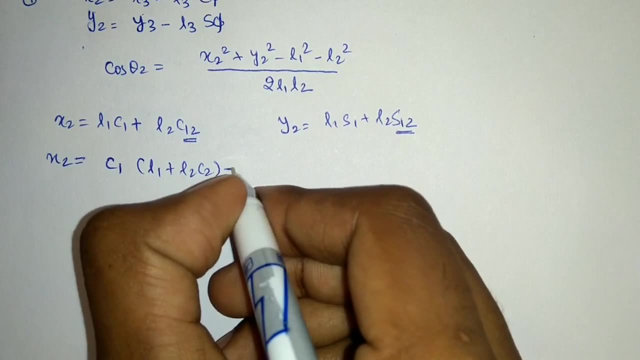 will apply the formula of s1- 2 here. ok, and I can get. x2 is equal to taking cos theta1, common c1 into l1 plus l2, c2 minus s1 into l2, s2- ok. at the same time, y2 will be equal. 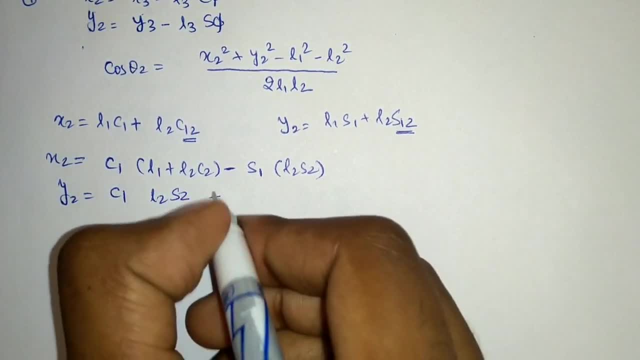 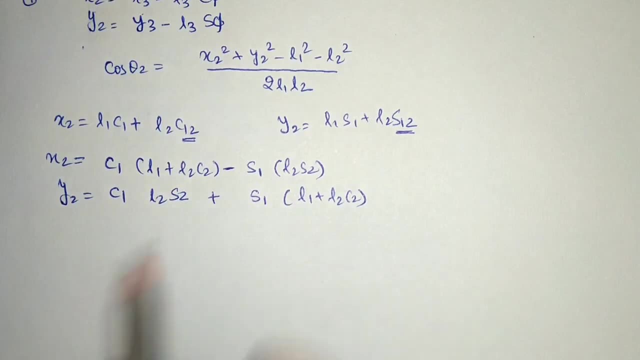 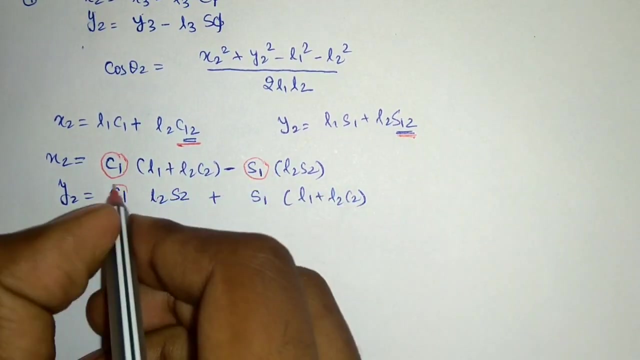 to c1 into l2, s2 plus s1 into l1 plus l2, c2. ok, this is just the expansion of these cos terms and sin terms, Ok, Ok. Cos theta1 common, sin theta1 here, cos theta1 here and sin theta1 common. ok, now I am having